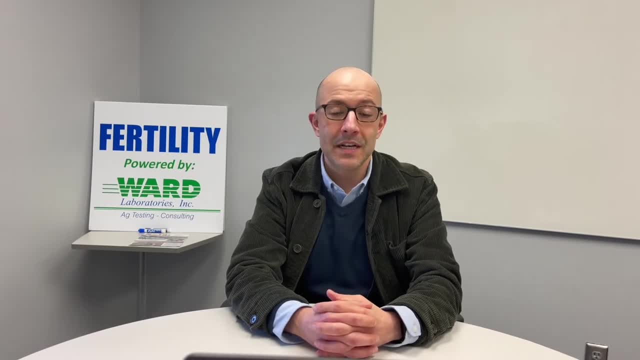 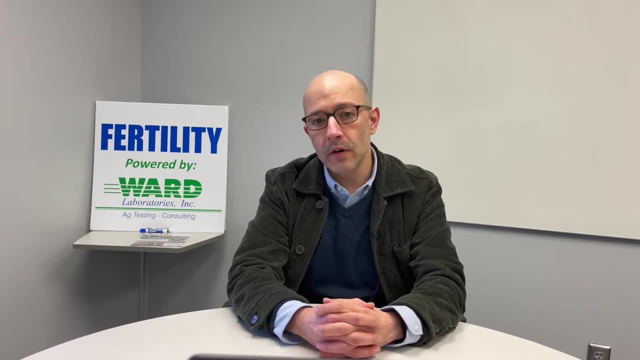 And a lot of that land was sold for development, And so we have many, many issues with this, or they're still growing things on them. So we have to look to see how to keep that arsenic and lead in the soil or remove it altogether. 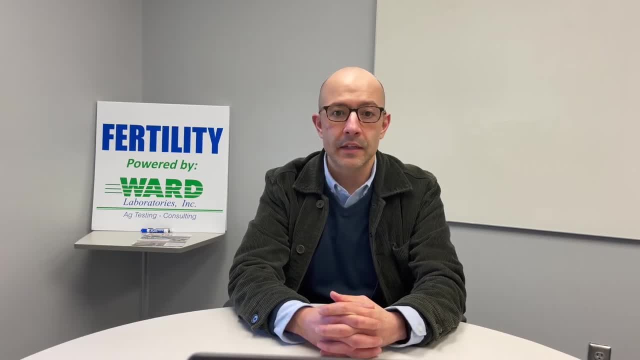 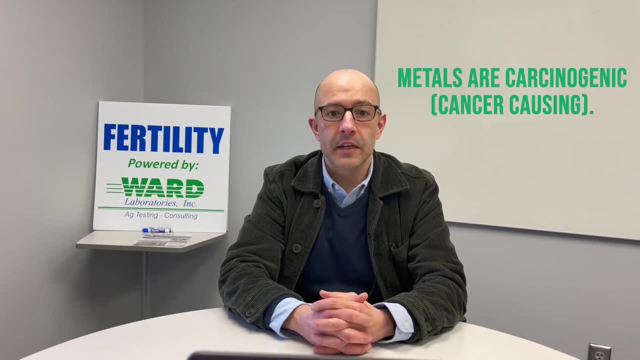 And not in the plants and the foods that we end up eating that are grown on those soils. So why are these a problem? So metals are carcinogenic. They're cancer causing for the most part, But one of the issues with lead is that it impairs child brain development. 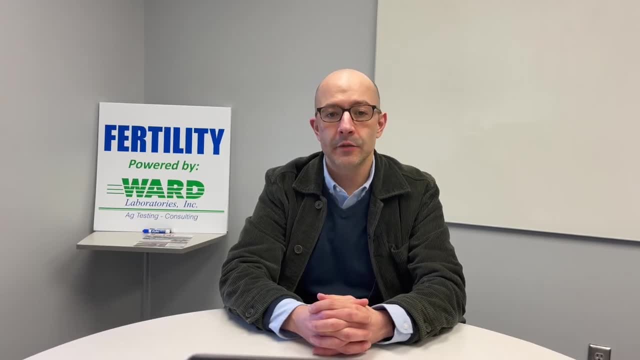 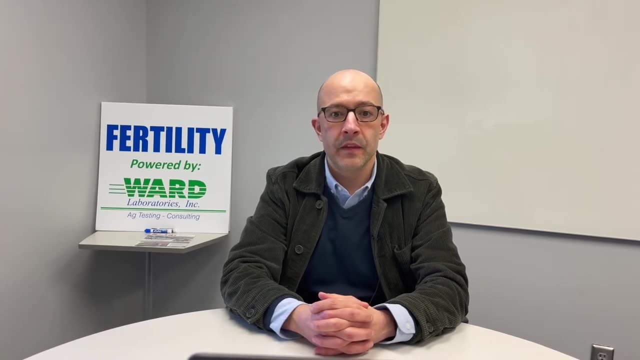 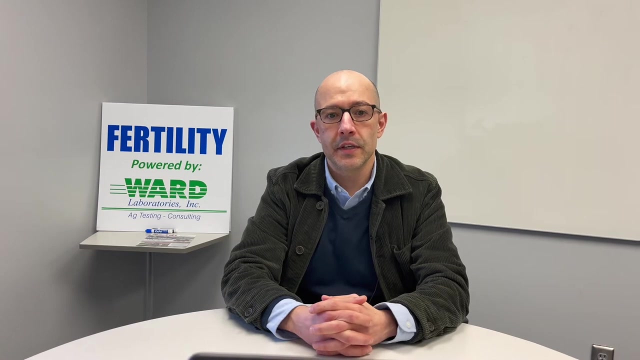 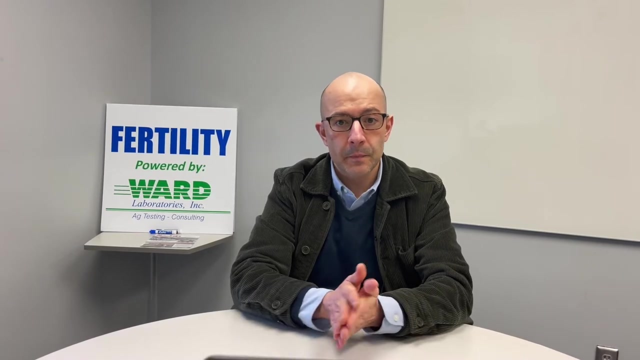 So keeping children away from lead exposure is a grave concern because they will be affected for the rest of their lives if they have physiological impairments from lead consumption. And arsenic and cadmium both cause cancer. So arsenic is very well known for causing skin cancers because it will degrade the keratins in your skin. 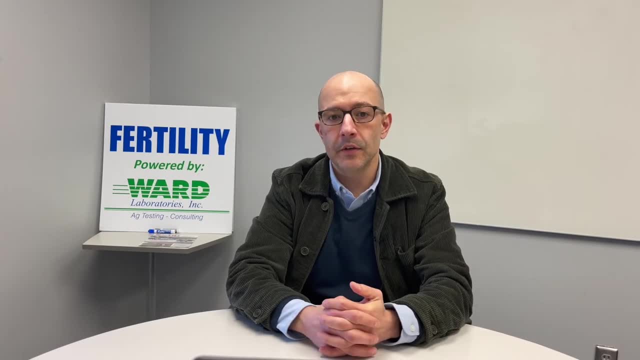 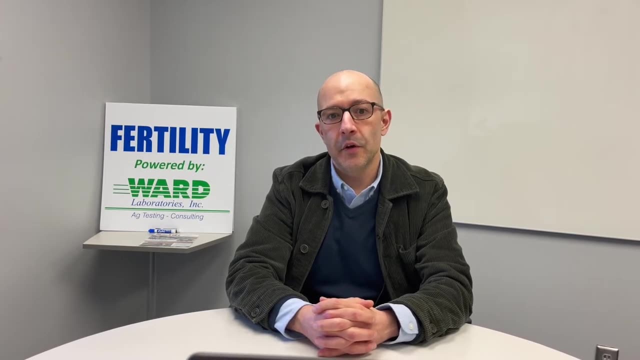 And then cadmium will actually replace, besides renal failure, which is the big cancer that it causes kidney cancer- it will actually replace calcium in your bones, And so it can serve the place of calcium, but not the function of calcium. So then the bones will eventually bend. 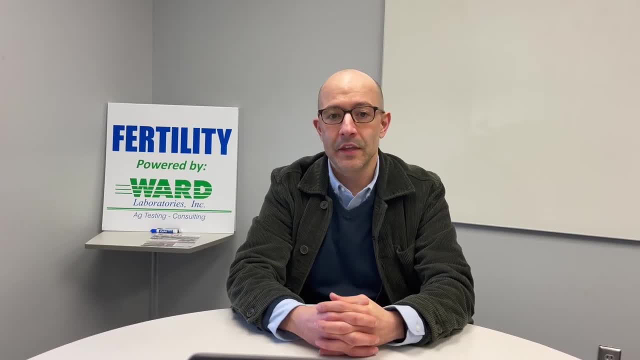 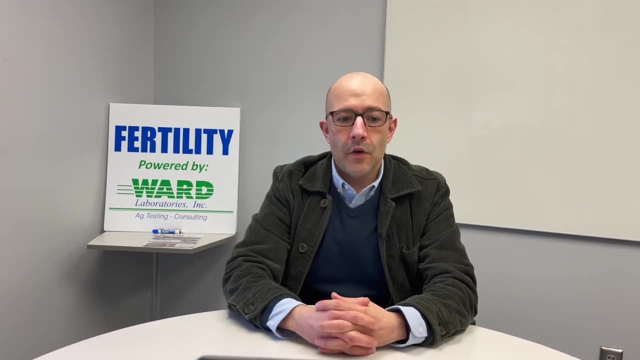 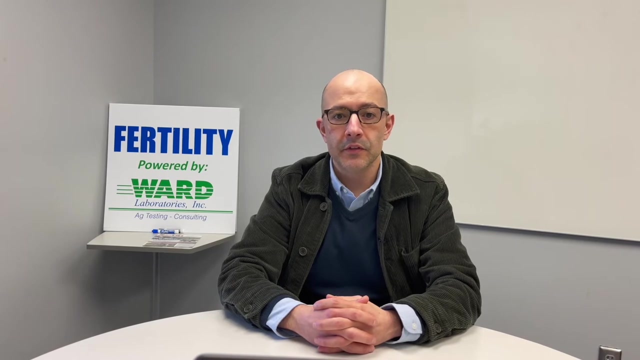 And lead will be affected And it will lose their support. So it's a huge issue with that. That's usually in places that have high amounts of cadmium in the soil, So typically other regions. So for the lead exposure risks in the environment, the EPA has given us guidelines for heavy metals in soils, especially agricultural soils. 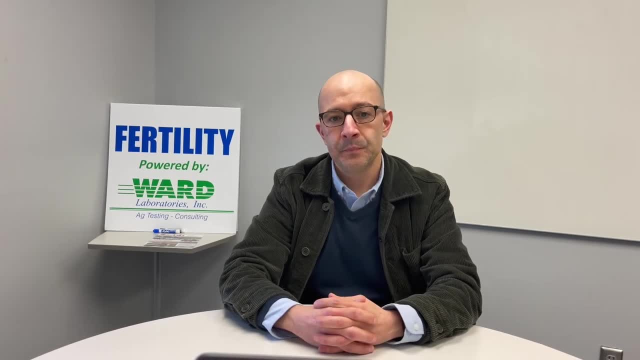 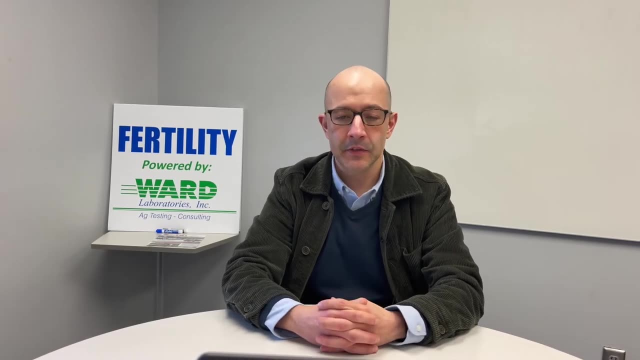 They have one for residential and then one for agriculture. the limits for these: They're much lower for agricultural soils, naturally, because we grow food on these soils and we don't want to eat metals. So for lead it's about 200 ppm in ag soils. 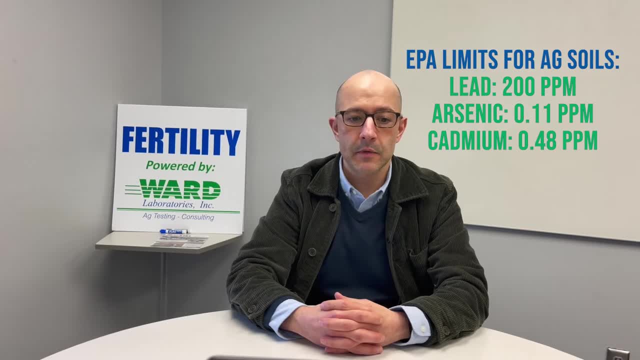 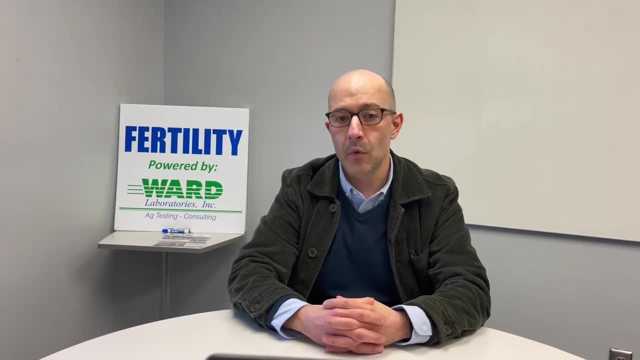 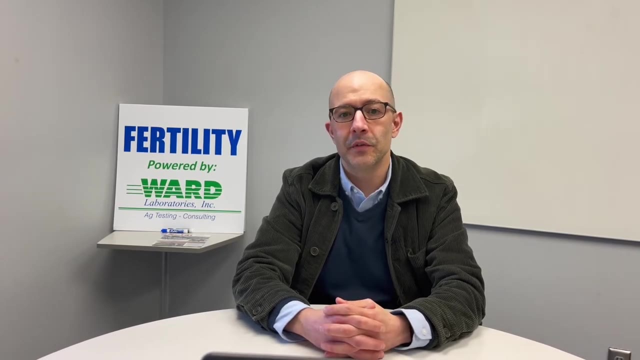 Arsenic is about 0.11 ppm And then cadmium is 0.48.. So it's quite low. And again, for residential soils they're much, much higher. I think for lead it's about 400, if it gives you an idea, mostly because no one's expected to eat the soil or really farm on those soils. 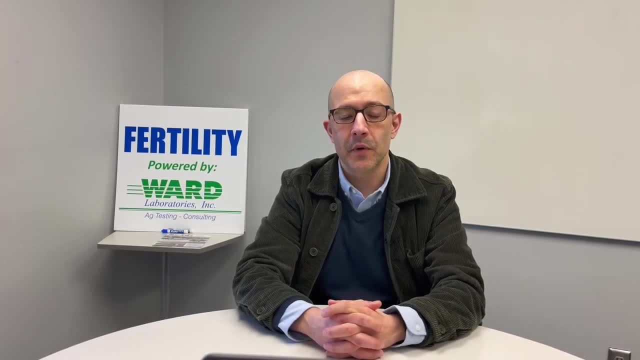 But you know, people grow gardens in their backyards, So we still get questions about this quite a bit. Some of the ways that the metals actually become very important is that they're not going to be used in the soil, So they're not going to be used in the soil. 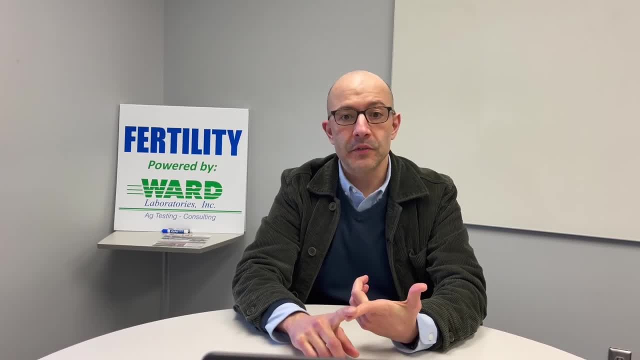 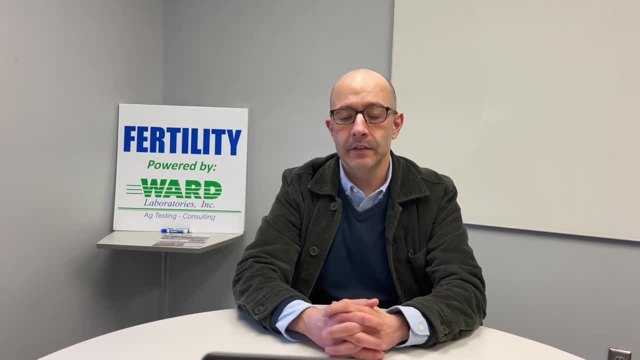 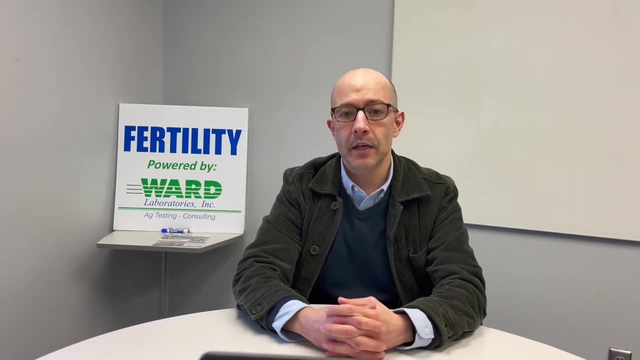 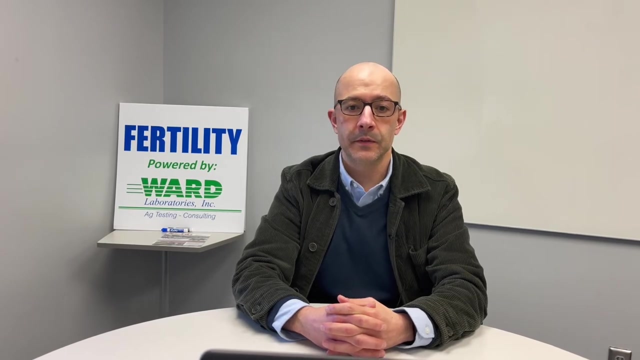 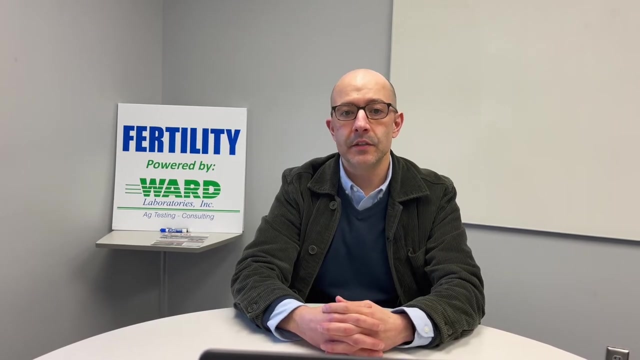 So tillage or development, things like that, industrial activity And rainwater. So rain events and wind events. wind will pick up the heavy metals and they'll increase their mobility in the environment and their ability to be taken up by plants, And then, with dust-carried heavy metals, we get exposed to that through inhalation. 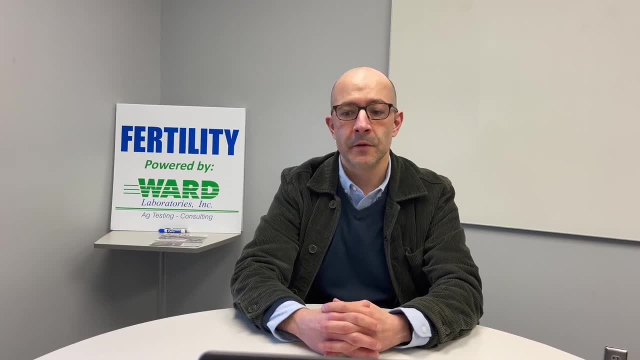 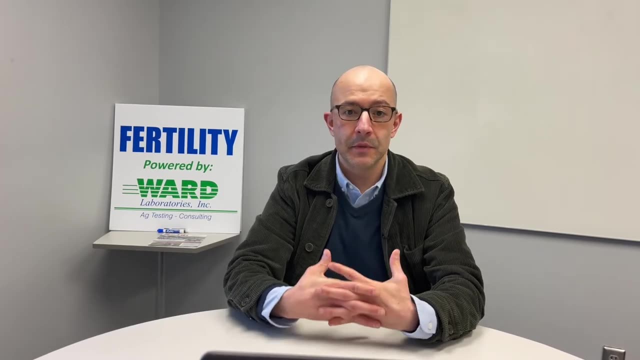 which is probably one, which is probably one worst ways to get heavy metals into your system, mostly because of the surface area of your lungs, Everything you breathe in is considered to be 100% bioavailable and, you know, assimilated into your, your physiology. so it's, it's. 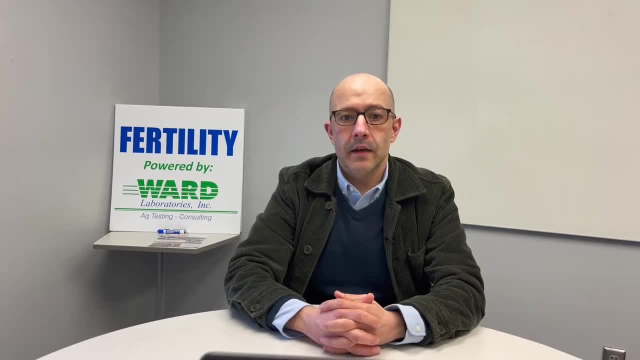 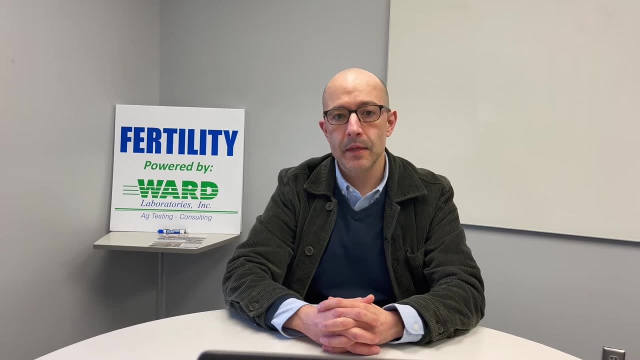 best to not breathe in heavy metals. So the uptake of heavy metals by plants is very crop specific and very metal specific. so to give you an idea, so for cadmium, some of the crops that are that are known to take up cadmium are lettuce. 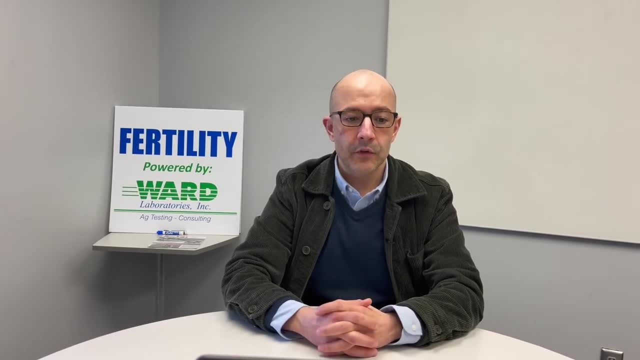 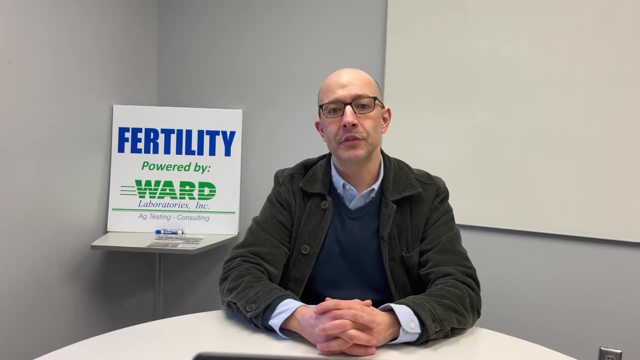 spinach, celery, cabbage and rice. For lead. lead's very. it's a very heavy or, I guess, a very large atom, so only a few crops can actually take it up. so kale, ryegrass and celery. There's probably a few other ones, but those are the main. 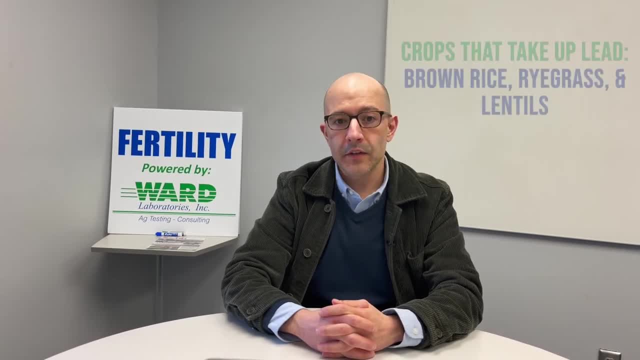 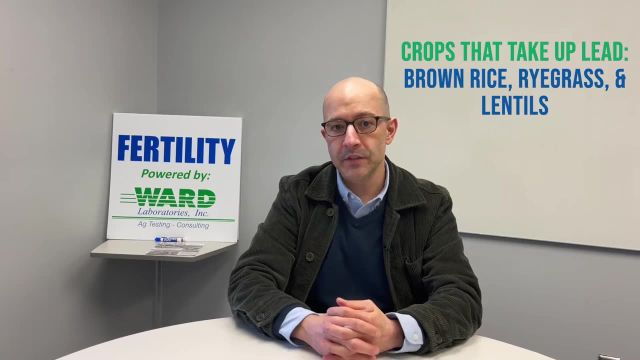 food crops. Then arsenic brown rice, long grain, dark rice- any rice with the brand the dark brand on it will take up arsenic and it accumulates in that brand. And then ryegrass and lentils are known to take up arsenic as well. 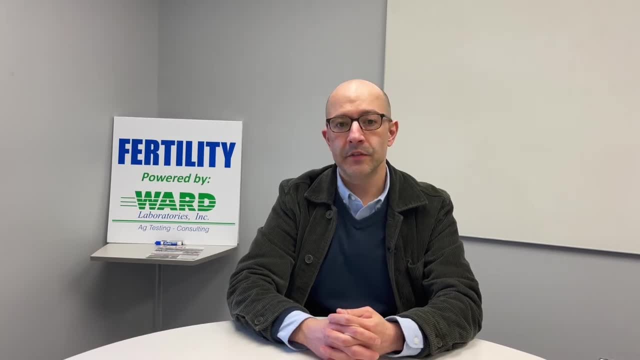 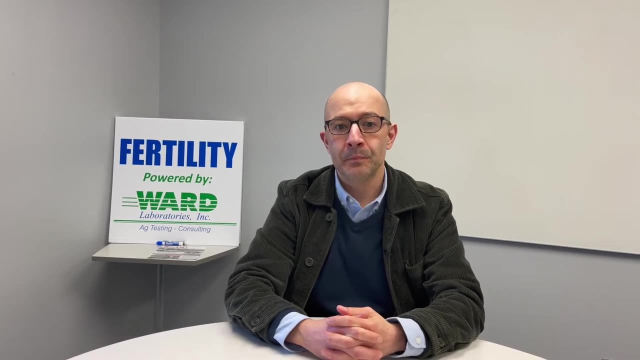 Rice also takes up a lot of these, mostly because it's a submerged crop and a lot of things come into solution and that sort of submerged aquatic system and the rice will just suck it up and put it right into the grain. so this is a huge issue in developing regions where they eat rice about four to five times a. 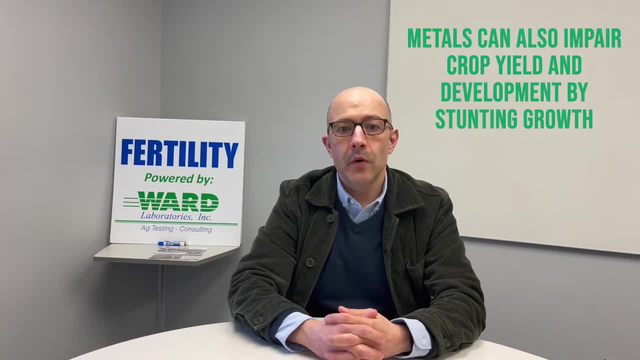 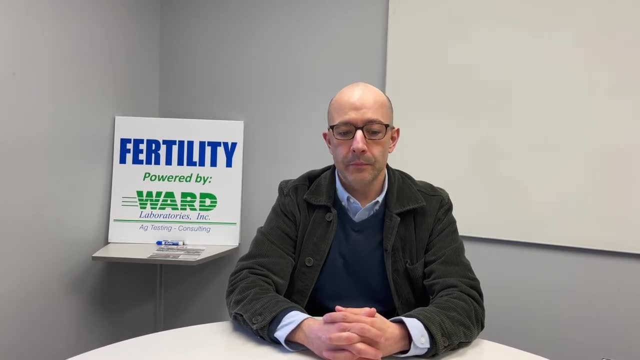 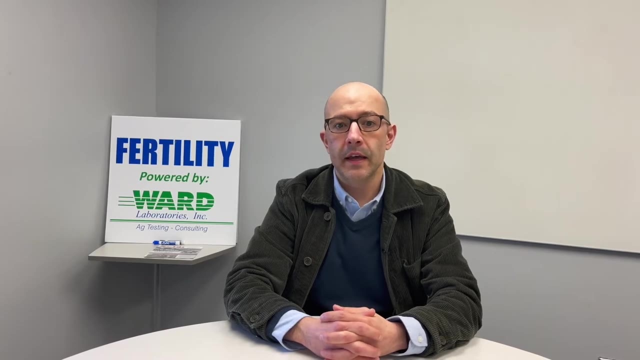 day. Heavy metals in the soils can also impair the crop yield and development, but those have to be quite high concentrations to do that. But usually if trying to diagnose issues in your crops and you've never done soil testing and you've sort of ruled everything else out, you might need to get a heavy metal sweep analysis of your soils just to see. 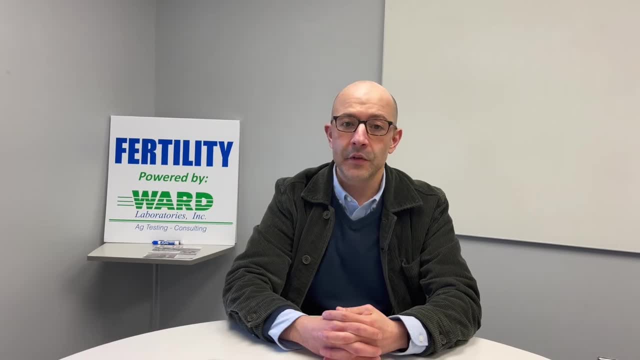 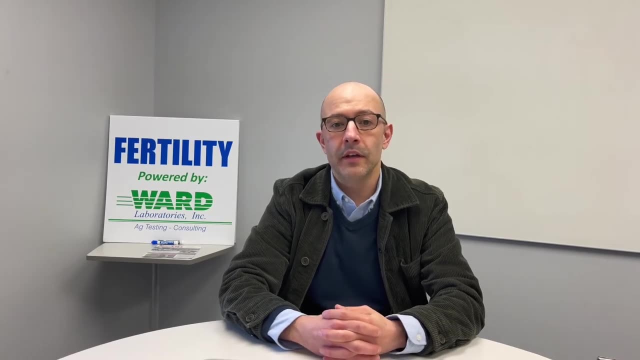 what, what's in there. that's usually a worst case scenario. it's also good to do that if you're, if you're, if you encounter a brand new field that you're working with, or even a new home, you know, if you're curious, if you want to do some gardening in your backyard, so just to be safe, especially in 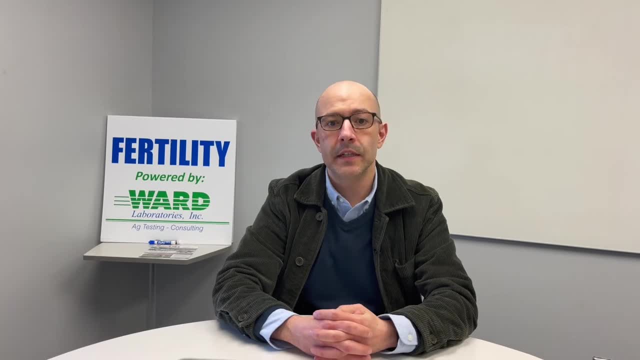 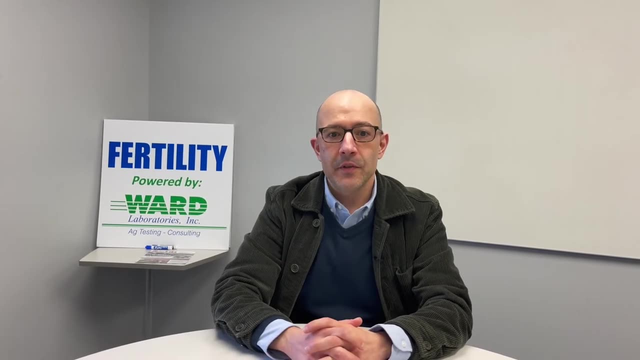 areas where you know that there has been sort of historic industrial activity or agricultural work that's been converted to residential areas. that's a really good thing to check out. there's a few other tests that we use that can actually what their function is: to sort of mimic, sort of 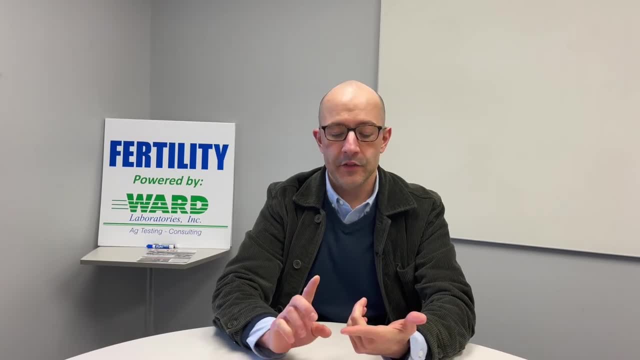 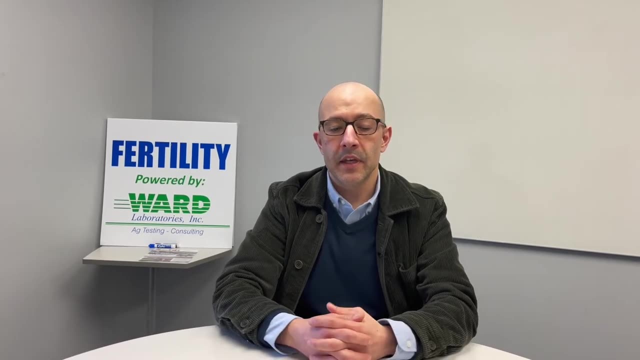 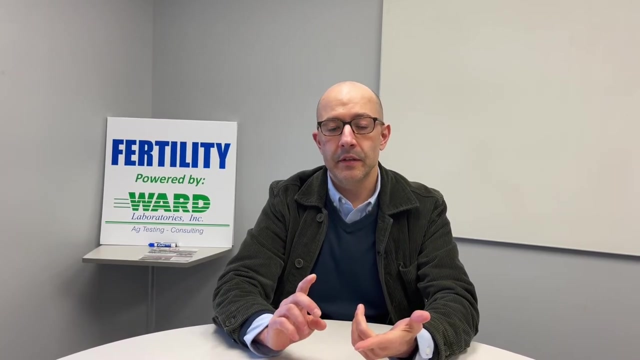 physiological systems, either in plants or humans. so there's one that mimics your gut that they applied to a lot of these metals to see how much is actually incorporated. the epa does some of these tests and there's some that we can actually do in a lab, even an ag testing lab, so we can use the, the micronutrient analysis. 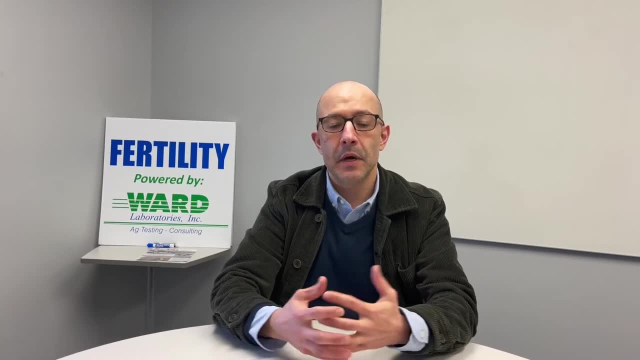 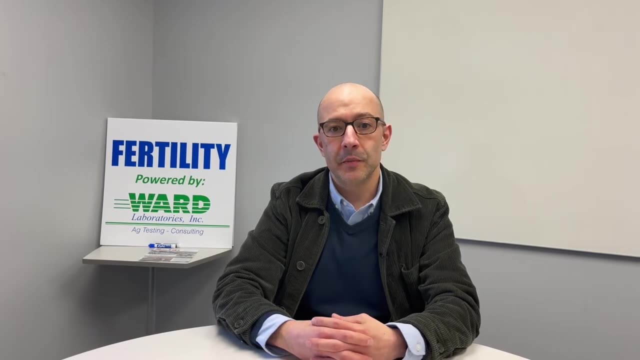 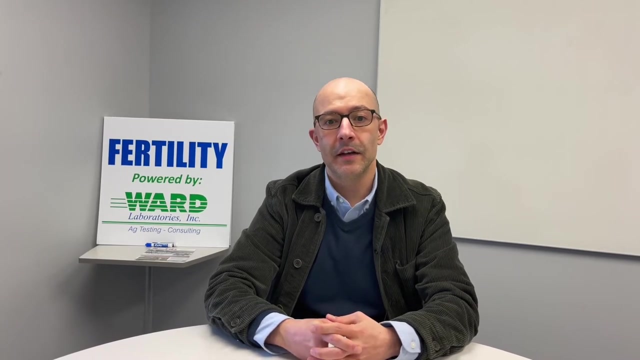 which acts as a plant chelator, which gives us an idea about the the plant available fraction. we can also use ammonium acetate, which is what we use for to determine your exchangeable nutrients, so calcium, magnesium, sodium, potassium. that also works as a plant available indicator. 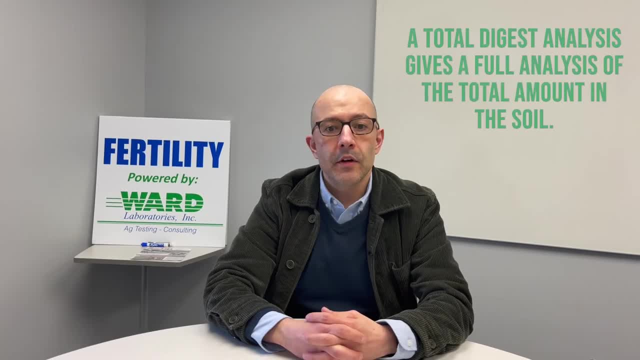 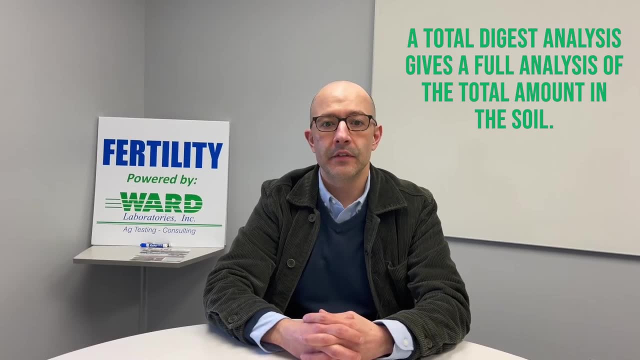 of heavy metals, and it's often used for that purpose. you can also do a total digest, which is what a lot of facilities do, which will give you a full analysis of the total amounts in your soil. it's a good to have that idea if you expect the concentrations to be. 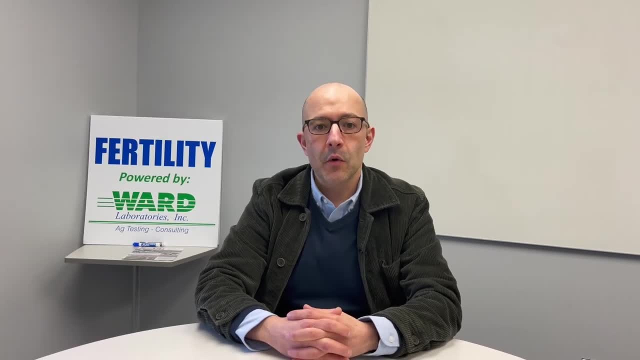 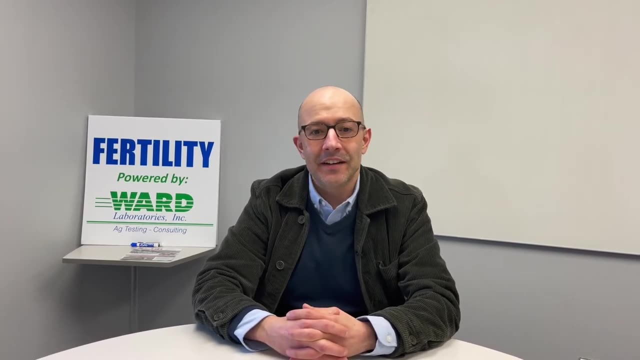 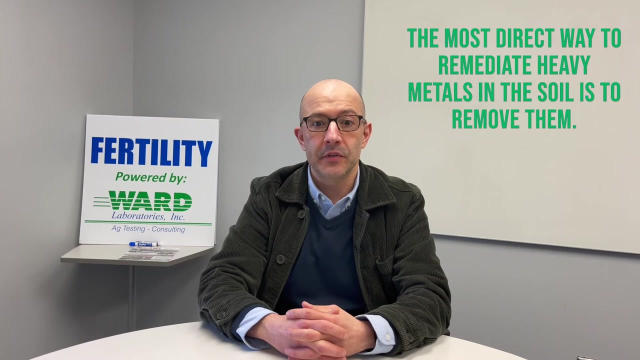 quite high. so the the most direct question we get- or I guess I get especially with doing this work- is: how do I fix it? so how do we get it out of our soil? the most direct way to remediate heavy metals in the soil is to just remove them. so topsoil removal and replacement, it really just depends on. 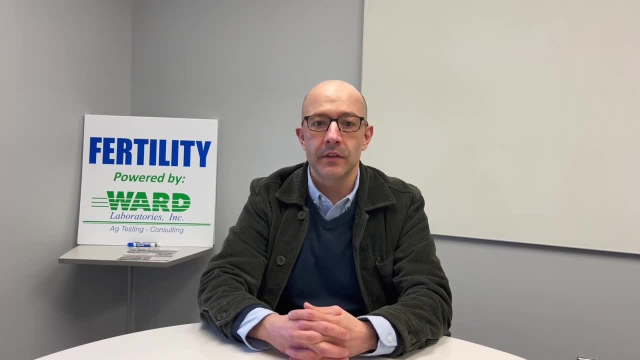 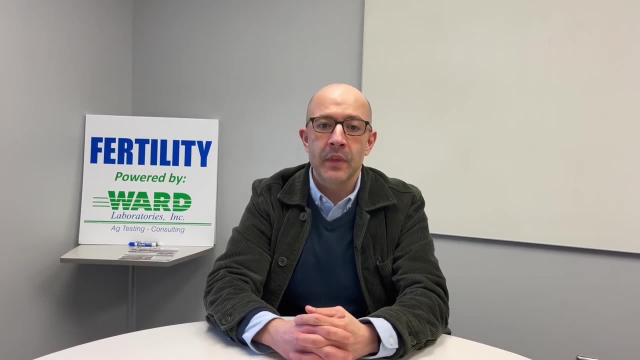 the concentration and the metal. like I said, not not everything in the soil is available for human or plant uptake. oh, it depends on the metal and the concentration and the form it's in in the soil. but if the concentration is quite high, especially in residential areas, usually the city will try to find. 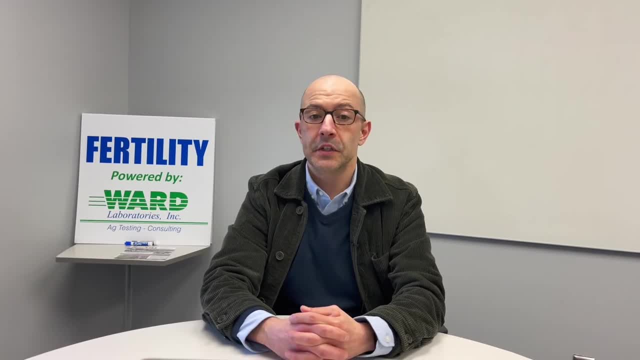 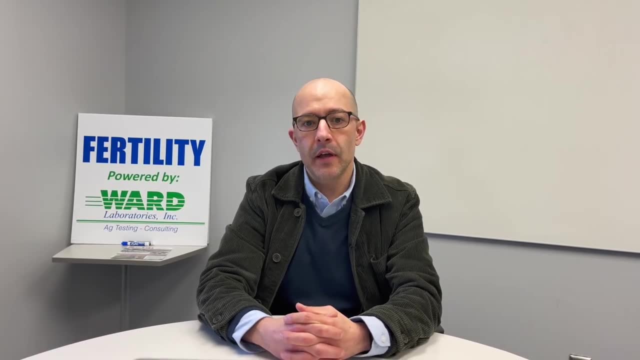 a way to remove it all together and replace it with fresh topsoil- fresh, clean topsoil. there's a few other ways to actually take care of the topsoil. if you want to take care of the topsoil, if you want to take care of this, so if you're, if you are near, like a untouched meadow or 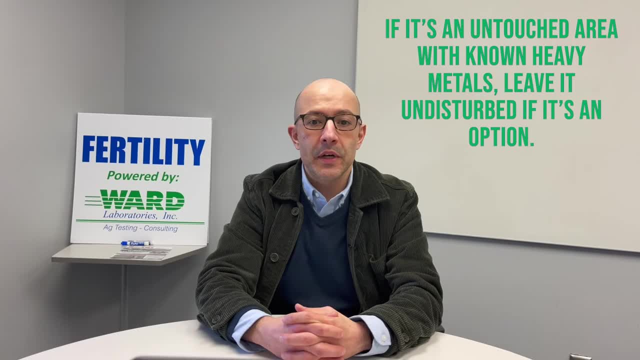 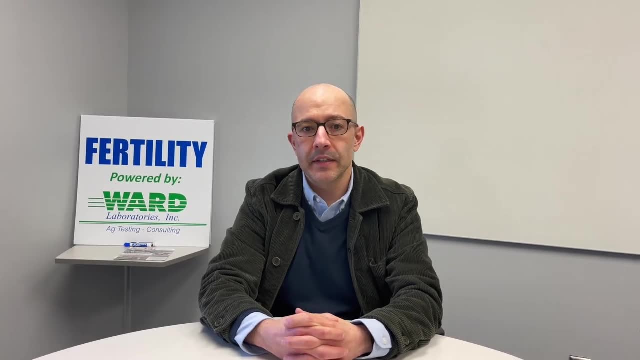 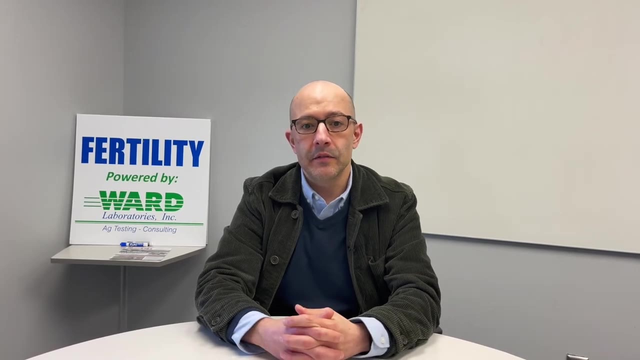 pasture and you know that there's heavy metals in there, just don't do anything with it. that's one option, you know. if you do have that option, and so don't graze it, because cattle can actually eat the grasses that are produced on there and don't farm anything on it or till the soil, don't disturb it or touch it. if 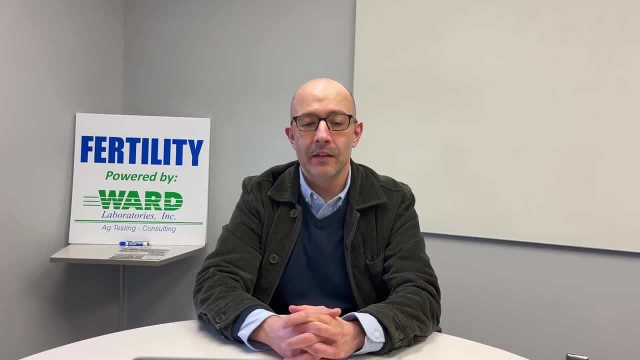 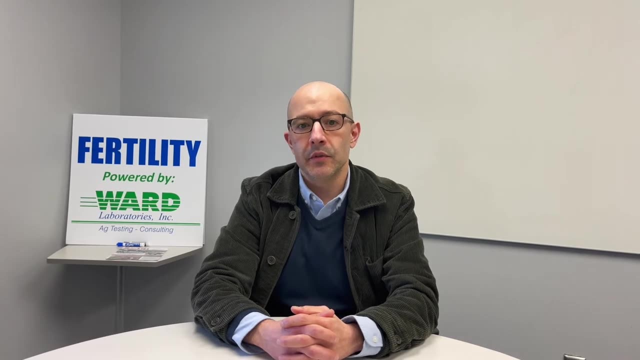 you have that option. now. a lot of people have a lot of land because they want to farm or Grey's cattle or something like that. so how do you remediate those soils to reduce the toxicity of those metals? there's a few amendments you can actually apply that have it historically been applied for a lot of these metals. 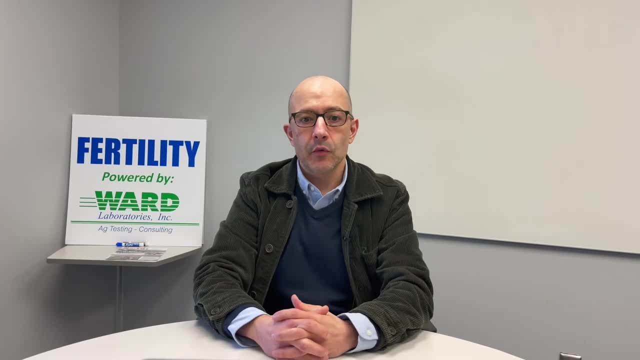 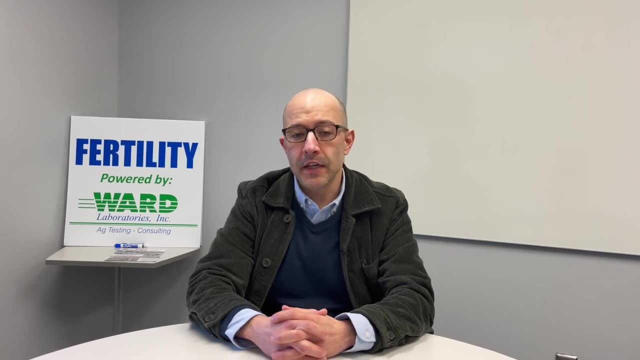 so some of these amendments that are used for soil remediation and contaminated soils- one of the most well-known ones is iron- iron-oxide, so especially for arsenic, iron. actually, if you think about, a lot of the planet is iron and so a lot of the 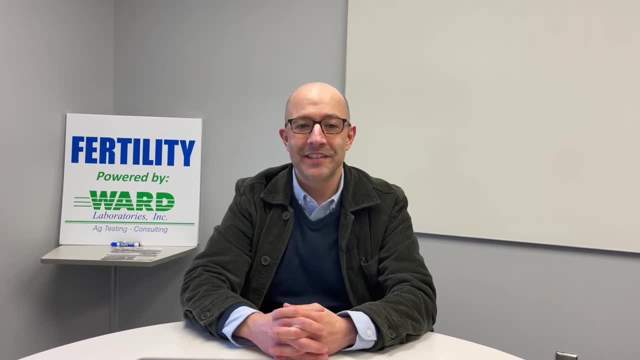 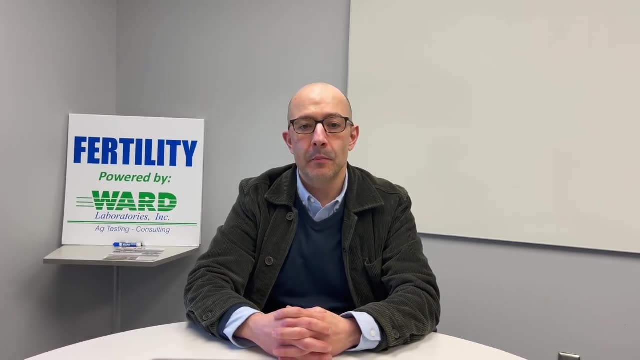 metals on our planet have a historic relationship with iron, you can say in a way, chemically speaking. but we use iron, we sort of exploit that relationship and apply it to help bind up and tie up some of these metals so that plants and animals won't eat them or consume them. 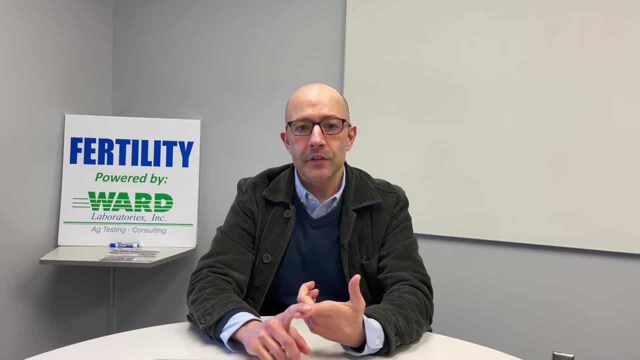 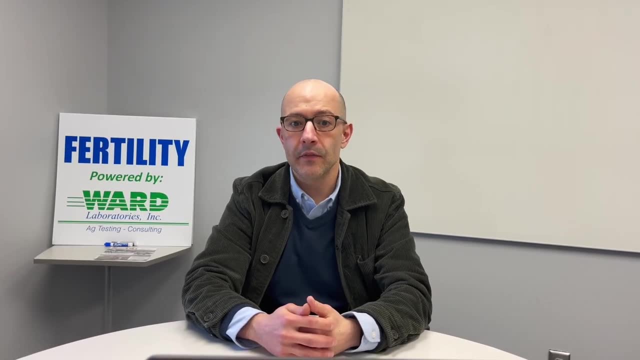 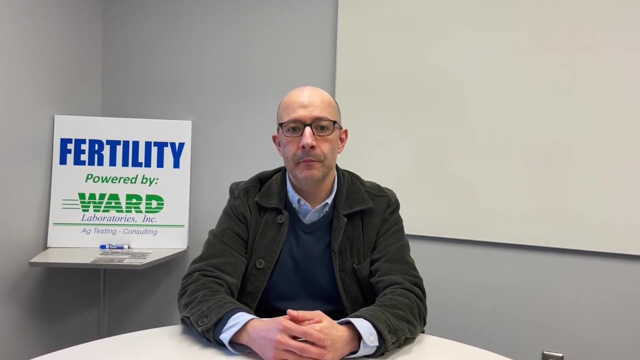 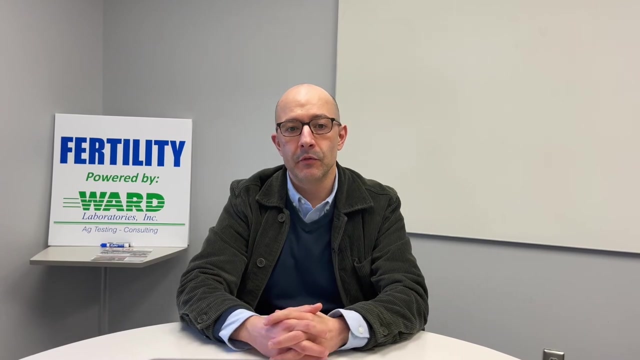 or take them up. so if you apply ferrous sulfate- which is a lot of what we apply for reducing- sometimes reducing the ph of soil, but also for iron availability issues, um iron chlorosis issues, we typically apply ferrous sulfate. we broadcast that about a half a percent by weight, along with a half a percent by weight of lime is, has been shown to be a really good way to remediate arsenic and soil. so that's a kind of a cheap, easy way to do it. you would need to test it out with some plants to see what's actually being taken up, have a test plot and then a sort of a control and a test plot to see what the differences actually are. so don't take it with. 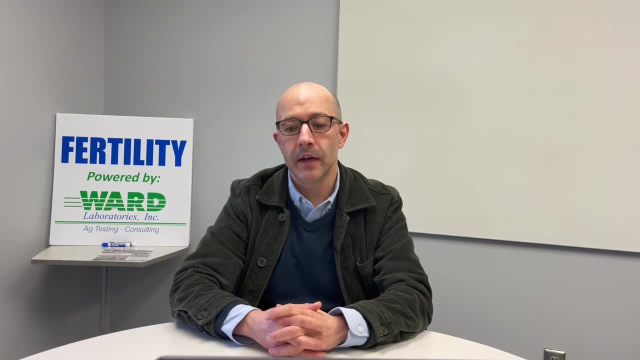 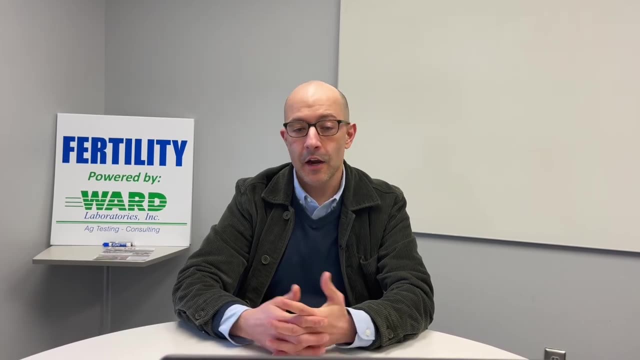 a grain of salt. you have to actually determine some of those for yourself and know the risks associated with taking that approach. that's you have to be quite clear about that, because it's not 100 curing the problem. you're just sort of changing the form in the soil lime itself has. 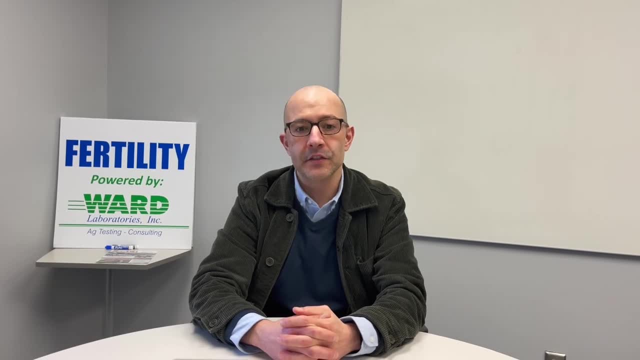 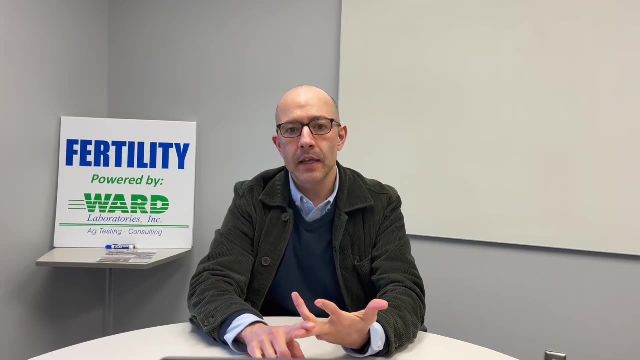 actually been used to remediate heavy metals in soils because you form these insoluble carbonate precipitates. so, and rice paddies, they've applied it for cadmium contamination. some people apply it for lead. it's not typically applied for arsenic, though, but if you raise the ph you'll typically change. 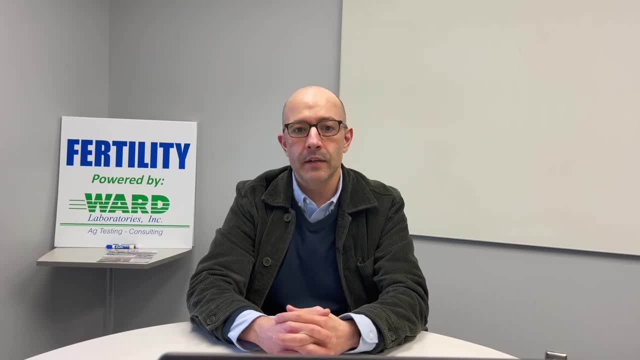 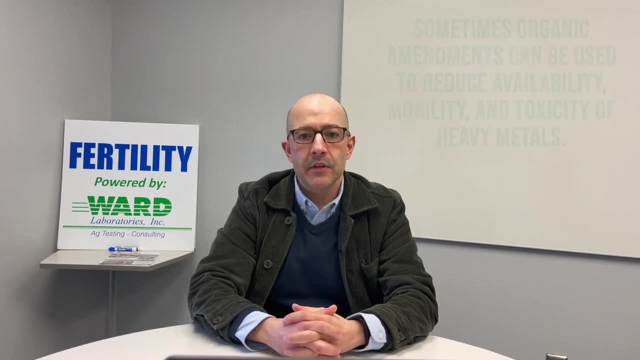 the form you'll precipitate things out and they're insoluble and not available for plant uptake. so that is also a very cheap option that people typically do in ag already. sometimes there's organic amendments that we can use to reduce the availability and mobility and toxicity. 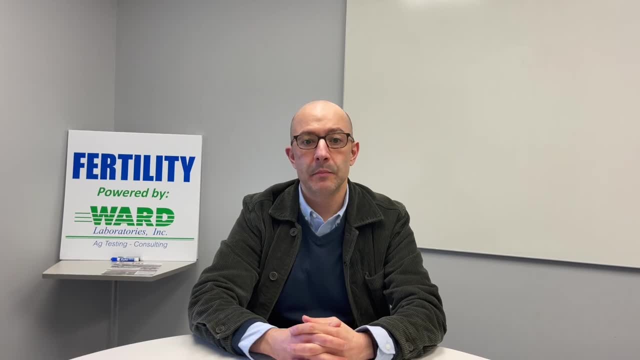 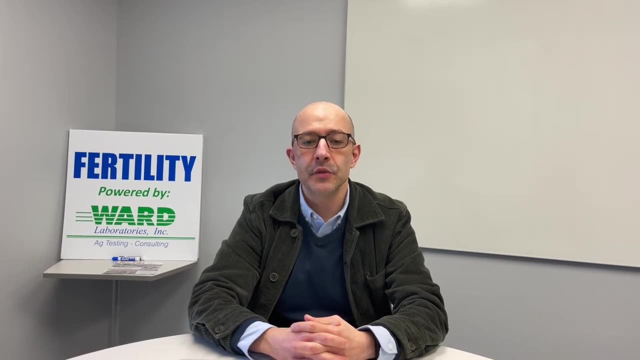 of some of these metals. so a very popular one recently has been biochar, which is just charred biomass. this is actually a pretty good option because you can use it to shower the crop and then you can take it off and you can leave it on your crop. 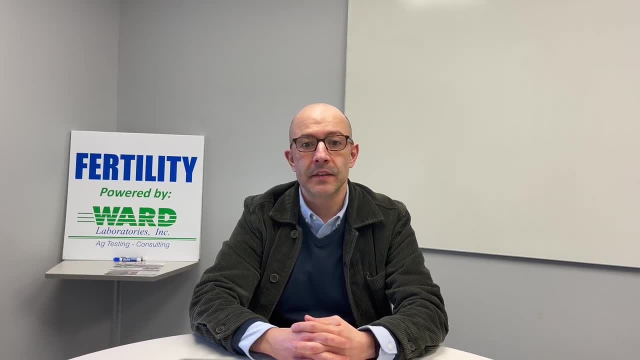 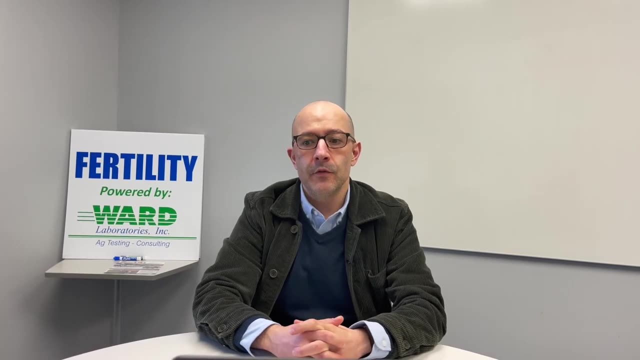 but there's a lot of people. unless you leave the residues on your crop, you typically have a lot of leftover residue and so people will take that you have to have a specific setup. so you're not, you know, ashing the material, you're just charring it a little bit and you form these. this really. 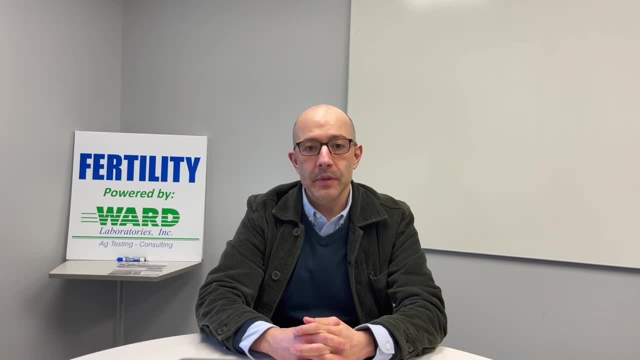 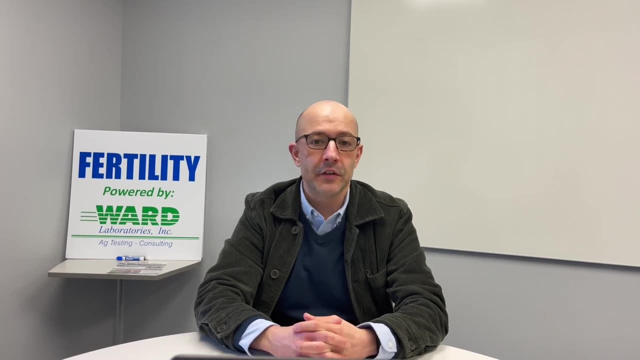 stable carbon sort of graphite material that you can apply and it binds quite readily to heavy metals, a range of heavy metals, which is pretty good. you can also mix that with some of the ferrous sulfate, and. And you can also mix that with some of the ferrous sulfate and. 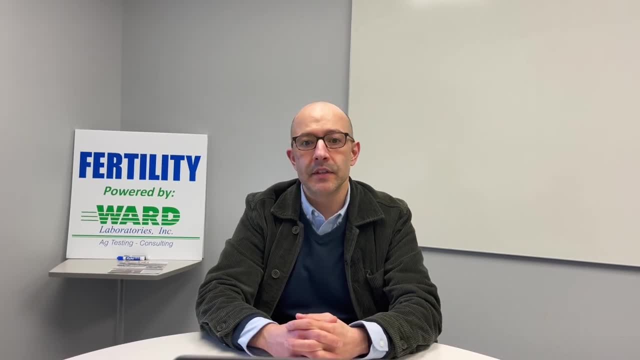 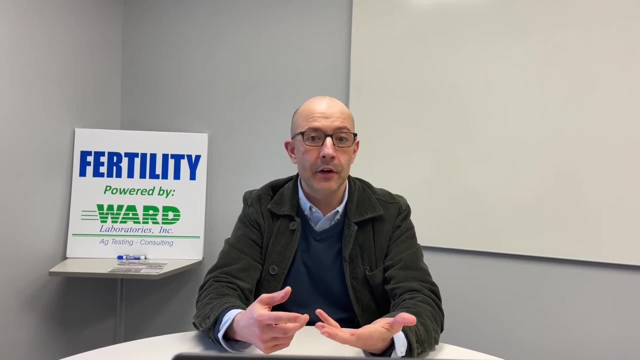 apply it and it forms a- I would say an- even more stable complex, because it not only gets some of the metals that it's known to tie up, but some of the metals that it's not really known to tie up, that typically the iron can get. so you, 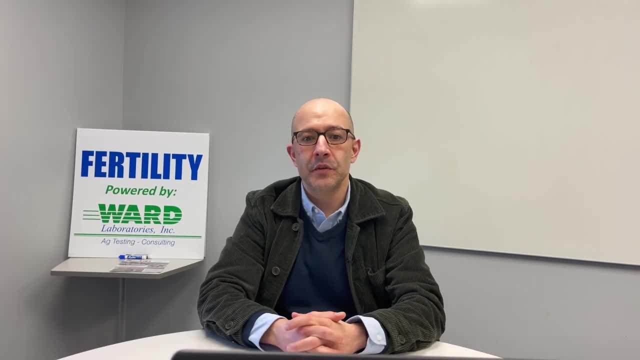 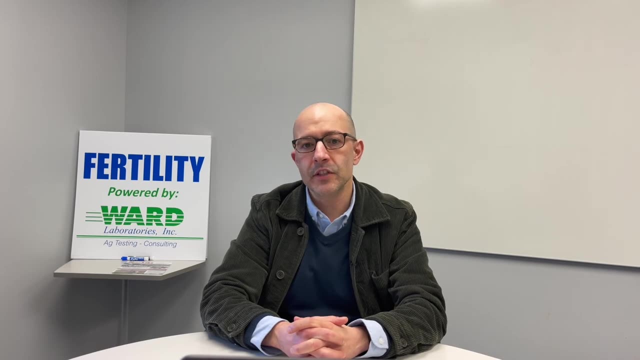 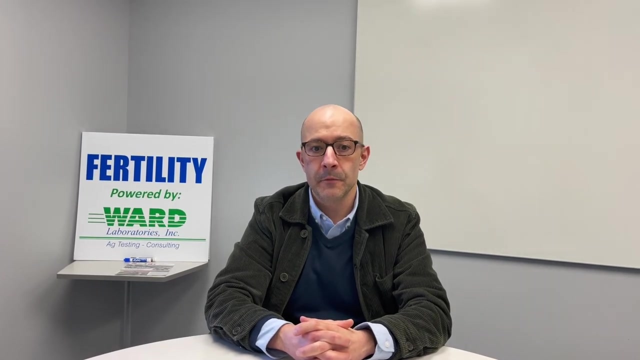 form this sort of whole. it's like a holistic approach to reducing the availability of heavy metals in your soil. you can apply things like compost, but it's only specific to metals like cadmium or lead and it has to be a very stable compost, so very well developed, not a young compost, because it's there's. 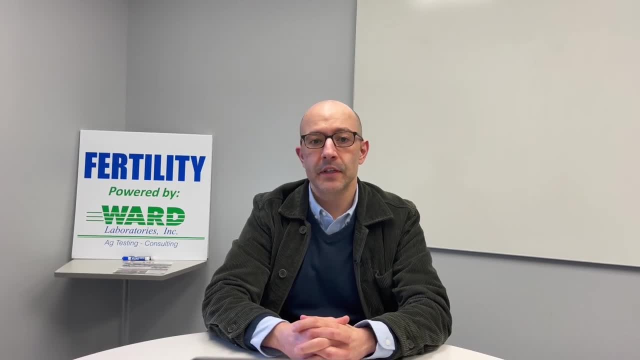 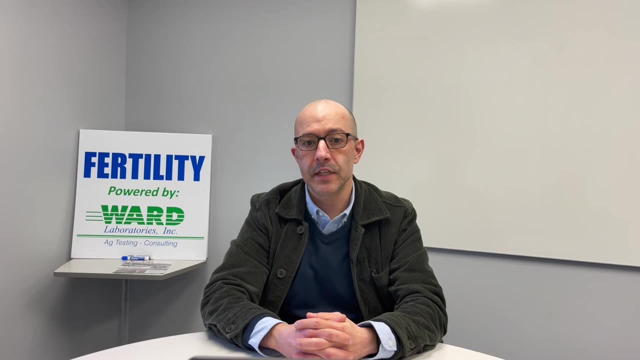 a lot of dissolved carbon that comes off the compost. that can actually tie up the lead and cadmium and make it more available for plant uptake or increase its mobility in the environment. so just keep that in mind. you have to kind of know the remedy for some of these metals in the environment you're not applying. 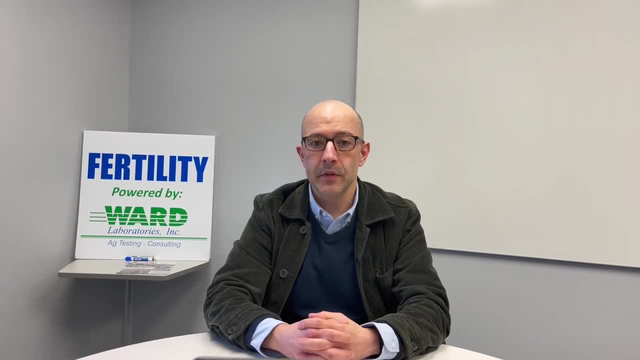 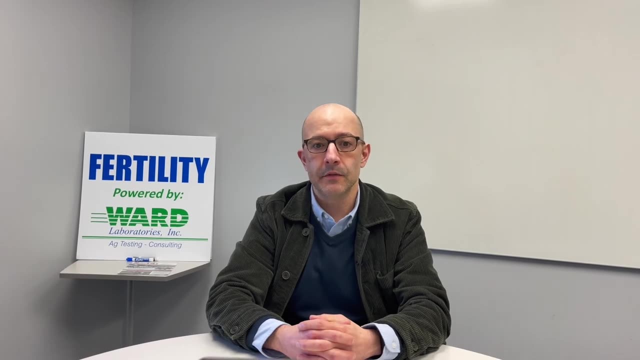 something that's going to increase the availability. one example is the application of phosphate for lead. it's been a lot of research and it's been a lot of research and it's been a lot of. it's been typically applied. it will for lead remediation because it'll form.